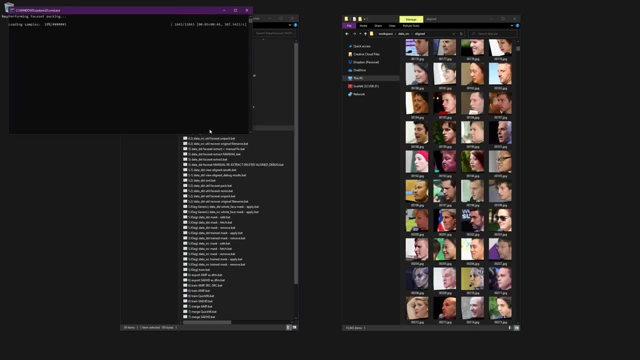 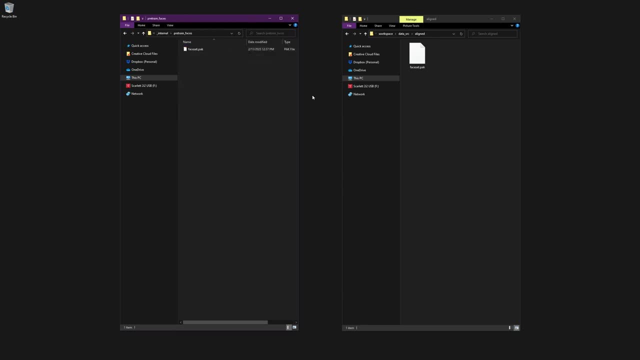 If you do want to use your own images, simply use the pack script. then drop the resulting face set dot pack file into the pre-trained faces folder, making sure to remove or rename the default face set first. Similarly, if you downloaded a pre-trained face set, just drop the dot pack file into that folder. 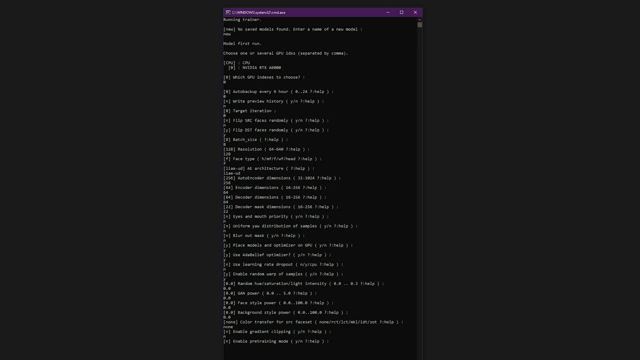 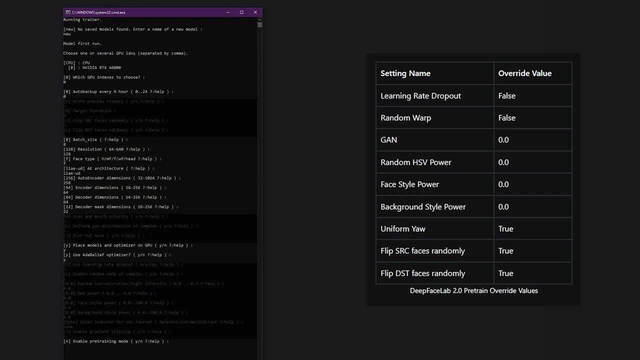 Now let's get into the model pre-trained settings. If you tried the SAE HD Trainer already, you may have been overwhelmed by the numerous options. Don't worry, because during pre-training we won't need to use most of these options and in fact the software will override several of them. 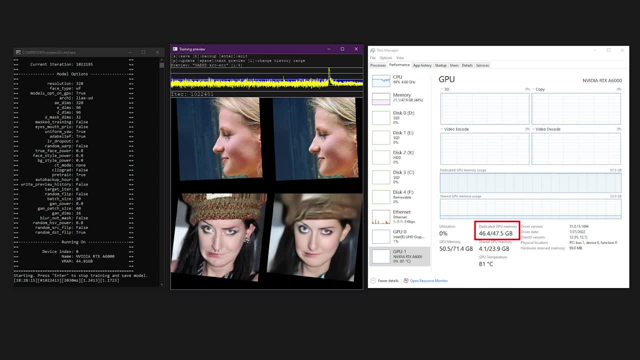 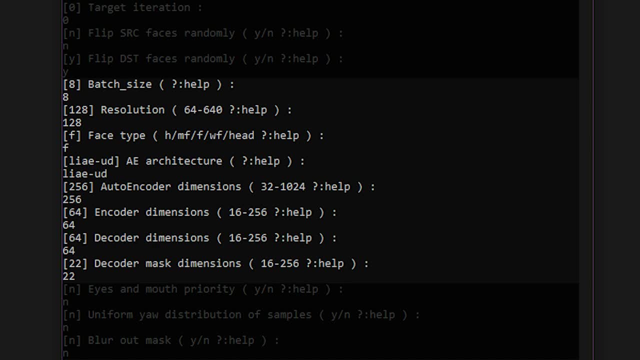 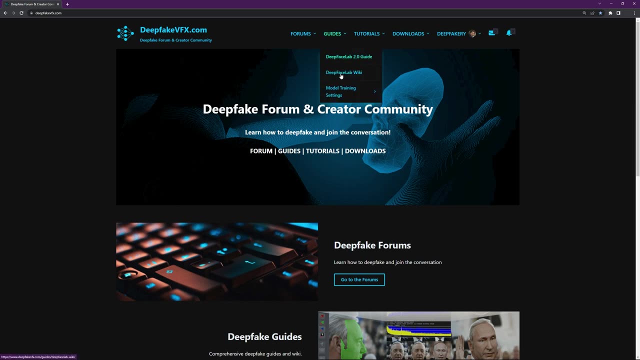 The goal here is to manage your VRAM and get the model trainer running on your system. For now, we'll focus on the main model architecture and parameters and I'll show you how to figure out what numbers to enter. Head over to deepfakevfxcom and, under Guides, go to Model Training Settings. 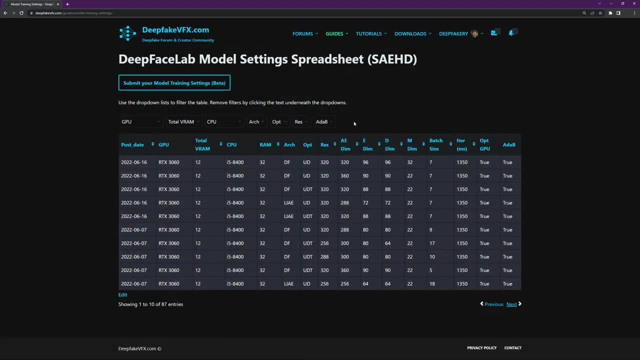 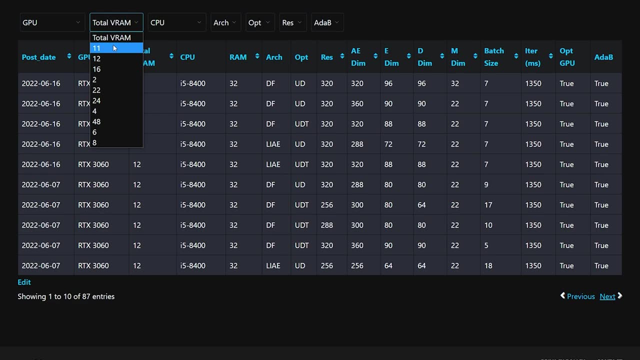 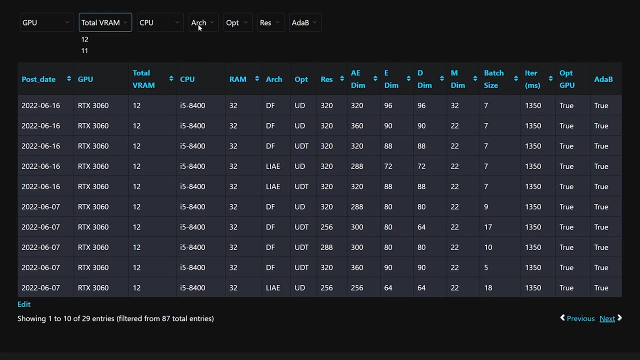 This table will help you choose settings suggested by other DeepFaceLab users that might work on your hardware. Start with the VRAM dropdown and choose the amount of VRAM that your GPU has, and maybe a couple of others. For instance, if you have an 11GB card, you might choose 11 and 12.. In this tutorial, 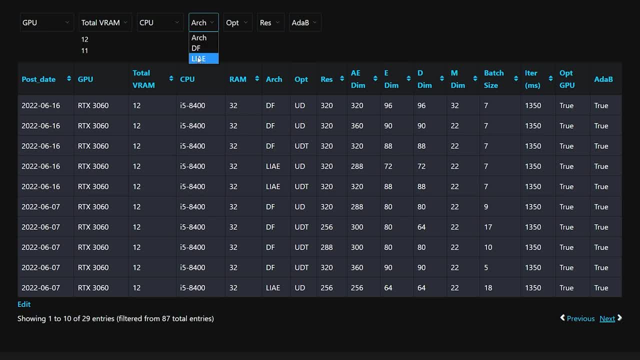 we'll be using the LIAE architecture, so you might select that option as well. These settings are merely suggestions and you can easily follow along by using the default values in the next section. Keep this window open and head back to your DeepFaceLab folder. 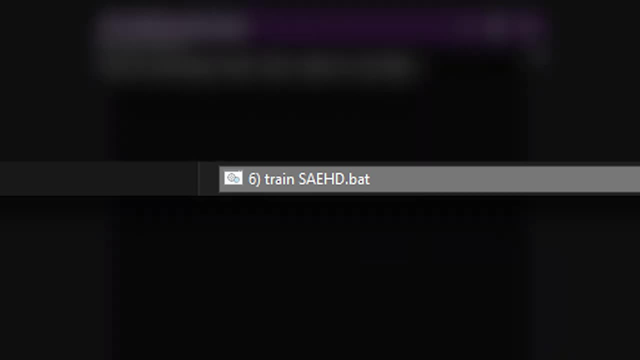 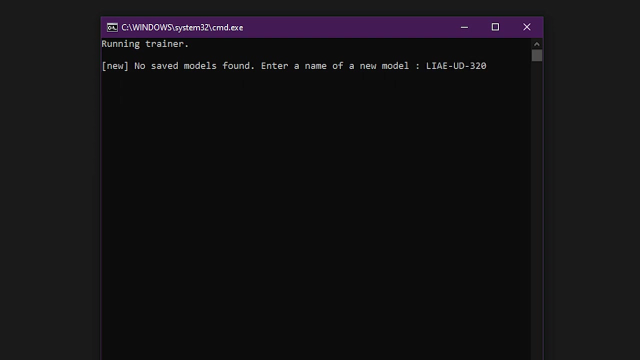 Now run the file labeled 6.trainSAEHDbat, The first thing you need to do is give the model a name. One naming convention you can follow is to include some of the model parameters in the name for easy reference. Keep it short and try to avoid using special characters or spaces. 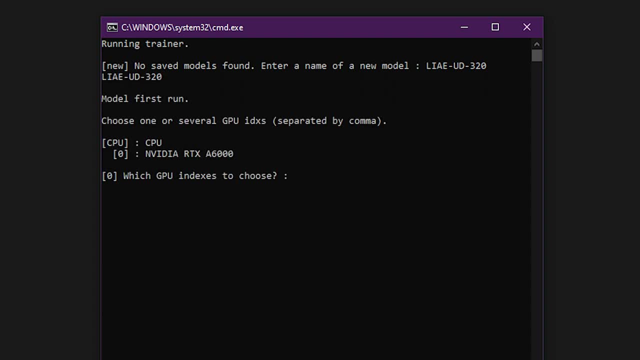 The next step is to choose your device from the list of CPUs and GPUs. You will probably be using the first GPU which is preselected as index 0, so just hit enter or type in the index of another device If you have multiple similar GPUs. 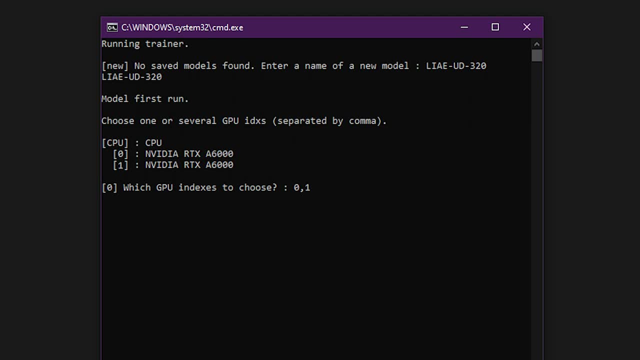 you can use both simultaneously by entering each index separated by a comma, like so: It is recommended that if you have multiple GPUs, they be of the same model or at least the same VRAM capacity. Also, note that you cannot combine CPU and GPU training together. We can set the auto. 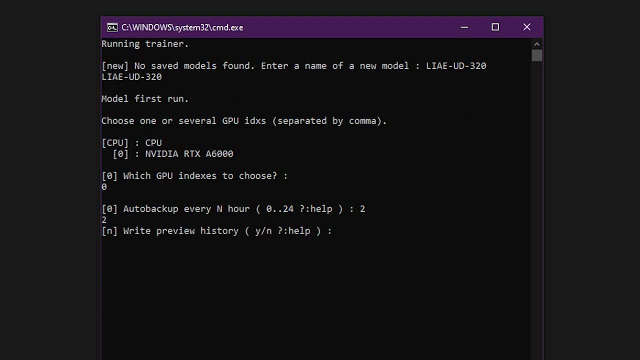 backup to 1 or 2, but that's up to you. If you have multiple GPUs, you can use one or more, Which one or two hours, and hit enter. Leave the right preview history at the default off setting. by pressing enter, You can set the target iteration to stop the training at a specific point or leave it. 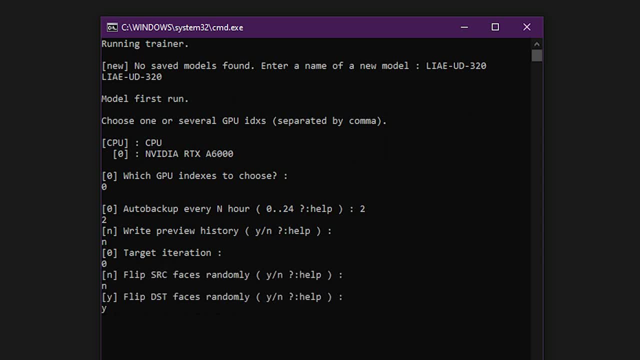 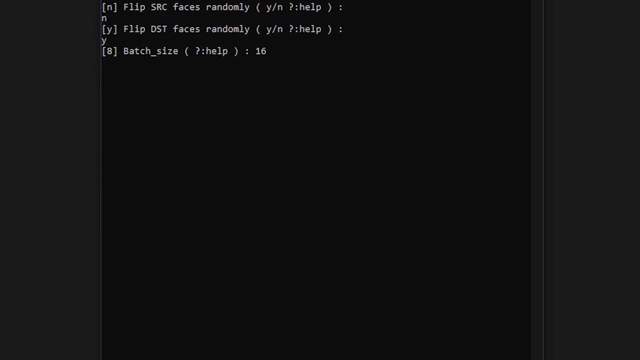 at zero for uninterrupted training. Flip source and flip destination randomly. can both be left at their default values. Now for the batch size, which sets how many images are to be processed per iteration. This is also the main setting that you can change throughout training to throttle. 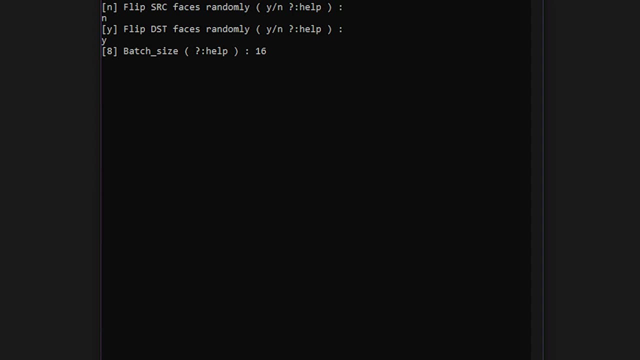 system resource usage to a stable level. Go back to the model settings table, if needed, and select one of the entries to use as your baseline settings from here on. Input the batch size listed there or, if you're unsure, just go with the default values. for now, The only caveat is that 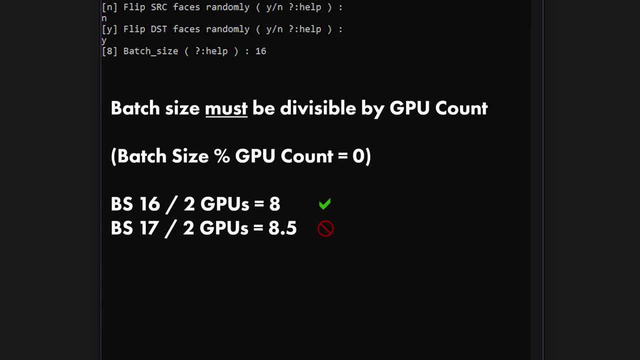 the batch size must be divisible evenly between all GPUs being used. For instance, if I had two GPUs, my batch size would always need to be an even number. If I had three GPUs, the batch size would need to be divisible evenly between all GPUs being used. If I had two GPUs, my batch size would always. 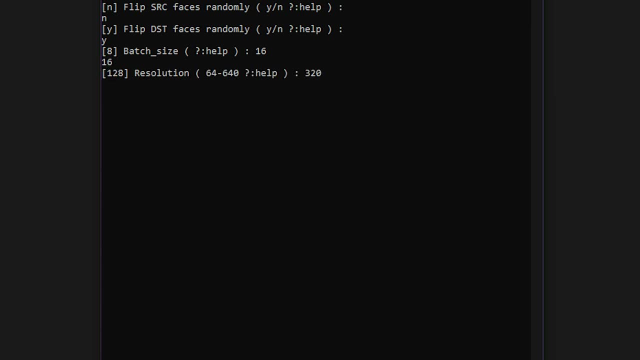 need to be an even number. If I had three GPUs, the batch size would need to be divisible evenly by 3, and so on. Next is the resolution, which is the main determining factor in the clarity of the resulting deepfig. Obviously, higher is better in most cases, but there's a limit to how much your 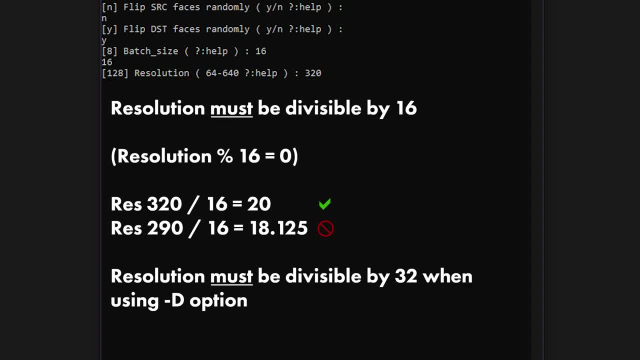 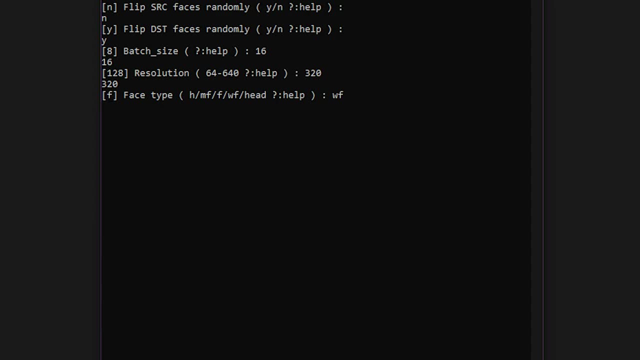 GPU can handle. Always choose a resolution that is divisible by 16 or by 32. if you are using the "-d architecture option, which we will get to in a moment, Enter the number from the table or hit enter to use the default. The face type is how much of the person's face will be considered. 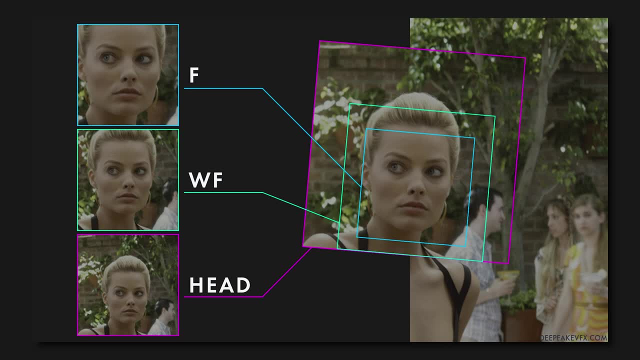 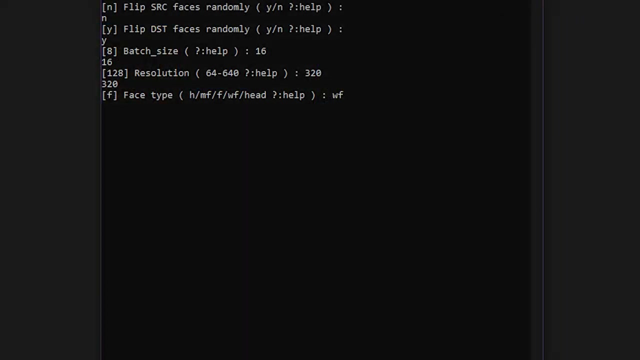 during training. Most people use WF, which stands for whole face. If you're not familiar with face types, please have a look at my face set extraction tutorial or the guide on deepfakevfxcom for a complete breakdown. Again, I recommend using WF. so type that in and hit enter. There are two. 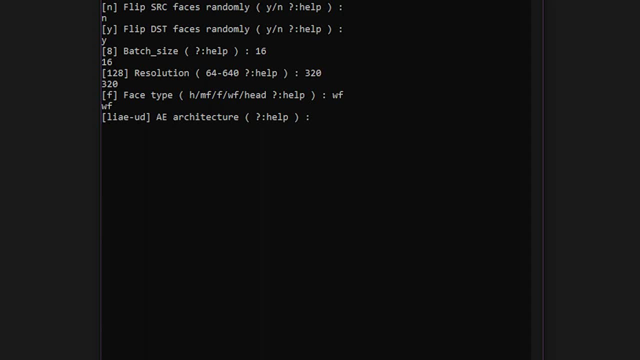 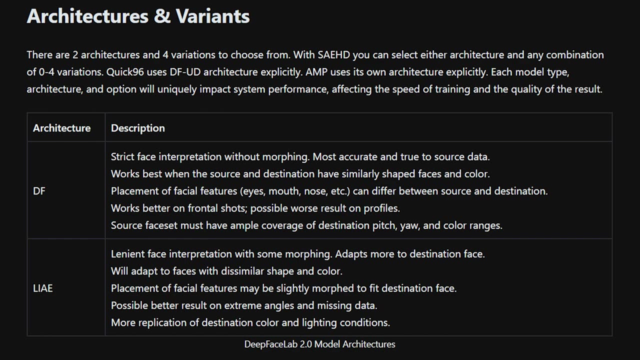 types of model architectures, as well as three standard options which you will combine: Df and Fx. Df is the original deepfake architecture and it tends to be more biased toward the source material. LIAE, on the other hand, has an easier time picking up the qualities of the destination images. 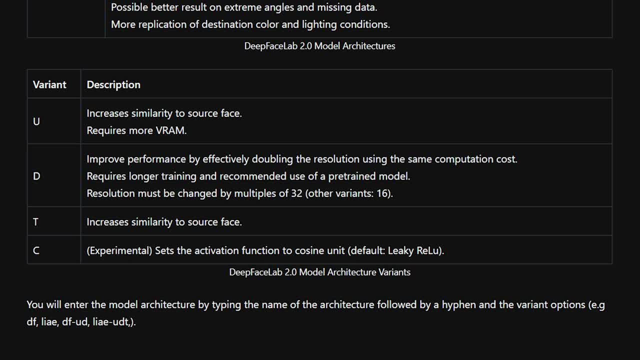 As for the options, you can add any of these to the model for a better result. However, you will be using more VRAM. when they are enabled, The U option increases similarity to the source, the D option doubles the resolution and the T option also increases. 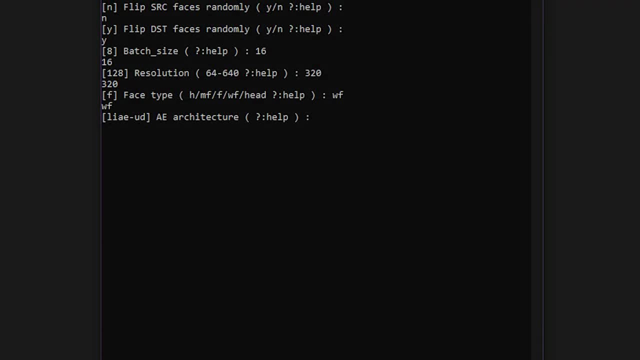 sources. The U option increases similarity to the source, the D option doubles the resolution and the T option also increases sources. I recommend entering LIAE, LIAE-U or LIAE-UD for the architecture type. The next group of options are used to define the dimensions of the autoencoder. 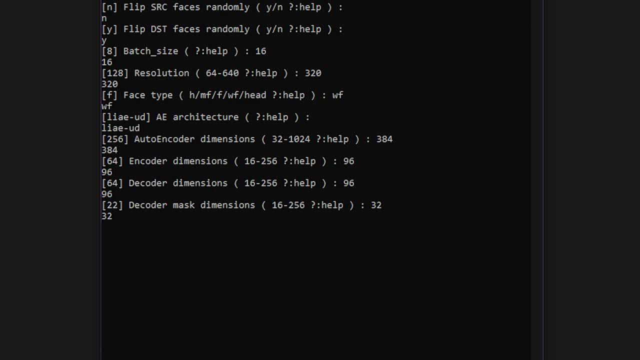 This is where things start to get a little more scientific, so I'm not going to go too deep on this. Frankly, if you want to know more, you're going to have to do your own research on autoencoders and neural networks In general. this affects the model's precision in detecting and 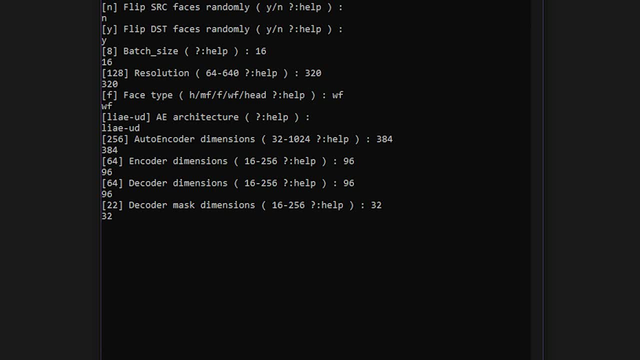 reproducing facial features, colors, etc. Here again, higher numbers are usually better, but they come at the expense of VRAM. Enter the numbers you found in the table or continue using the defaults. Mask training, eyes and mouth priority uniform yaw and blur out mask. can. 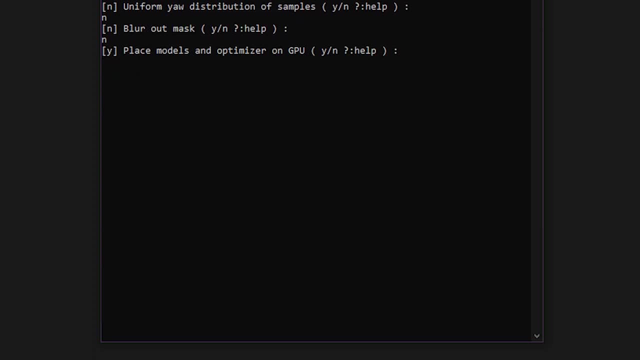 all use the default values by pressing enter. Model and optimizers on GPU may come into play later if you can't run the model, but we'll leave it on for now. Add a belief is what's called an optimizer, but what you really need to know is that this might make your deepfake look better. 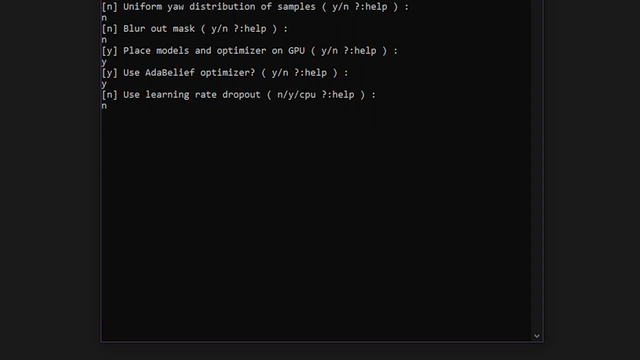 while again using more VRAM. Leave it on for now. Learning rate dropout, random warp, random HSL GAN style powers, color transfer mode and gradient clipping can all be kept at the default values. Finally, of course, we will enable pre-train mode. Now comes the moment of truth. Either 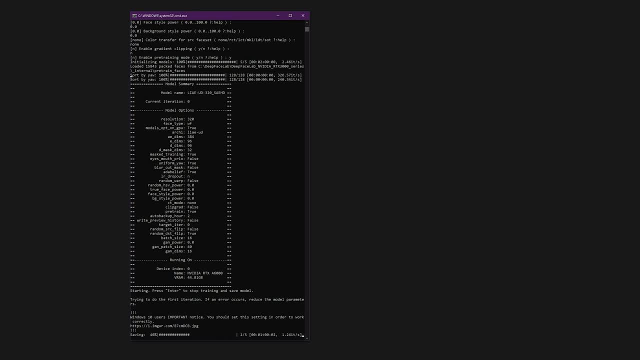 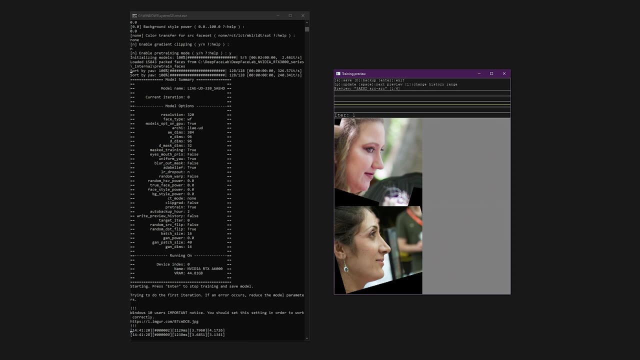 the training window will open or you'll get an error, most likely an out of memory or OOM error. If your model crashes, I'll explain what to do in the following section. Let's have a quick look at the SAE HD Trainer interface. 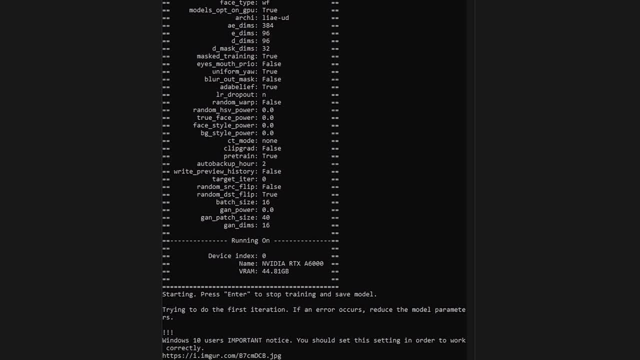 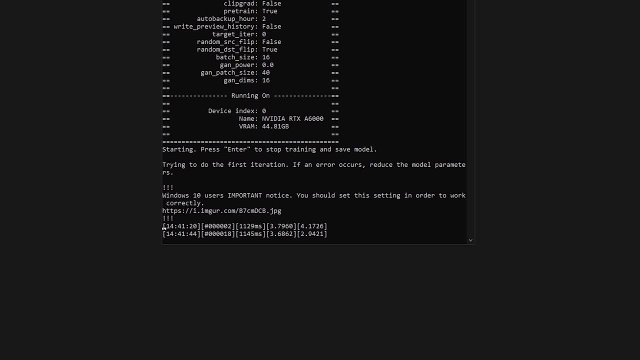 In the command prompt window you'll see the model summary which shows all of the settings you entered. Please note that the settings which have an override value during pre-training will not display the current values. At the bottom of the window are some sets of numbers which will show. 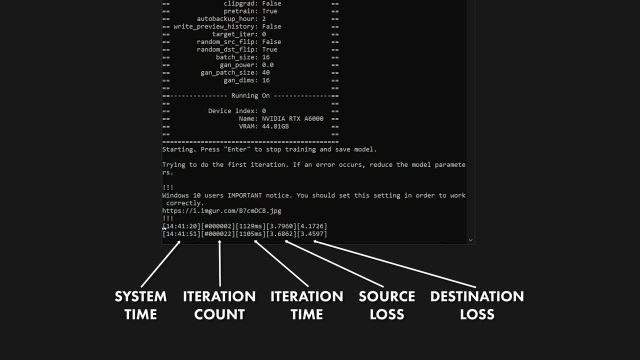 the model training progress From left to right. these are the system time, the current iteration time to process the current iteration, the source loss value and the destination loss value. These loss values represent the accuracy of the training and will approach zero over time. 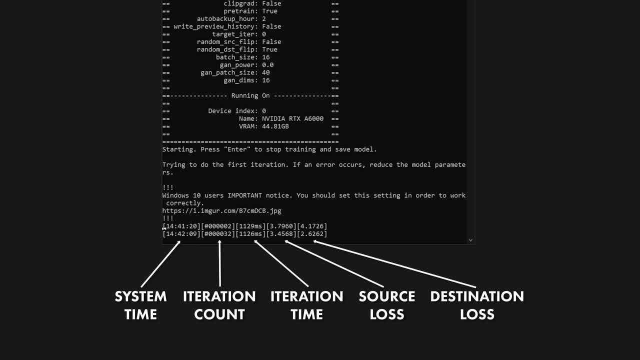 so the lower the value, the better the result should be. These numbers will continually be updated as the training progresses, but if the numbers stop updating, that means the trainer has frozen and will likely crash. The training preview window shows a list of commands. 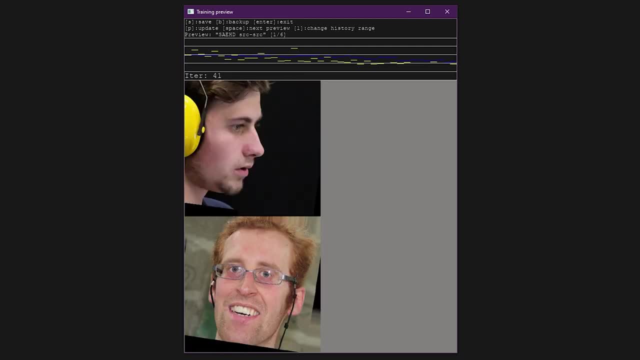 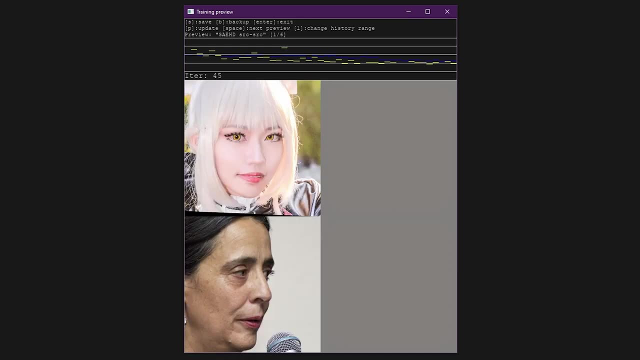 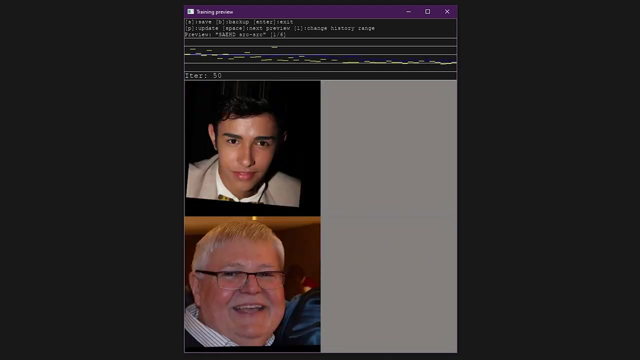 a graph of loss values and a preview image of the training process. You can save or back up the training or hit enter to stop training. You can easily restart training at any time by running the trainSAEHD script again If you would like to refresh the preview image. 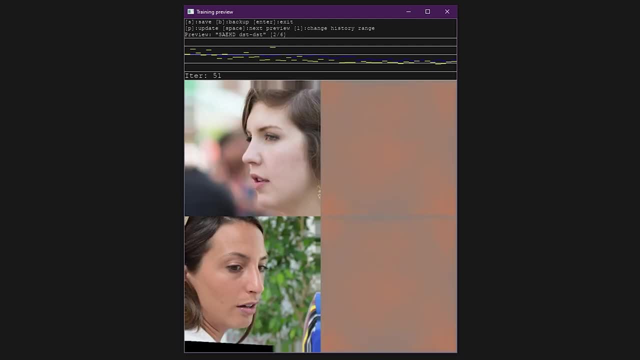 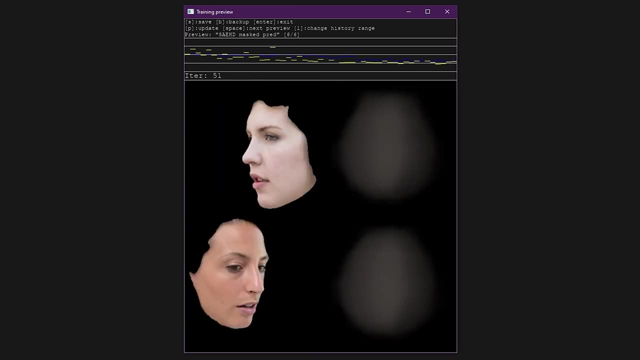 press the P key to update The spacebar cycles through preview modes showing masked and unmasked versions. The L key changes the range history of the graph, which will be helpful as the model reaches maximum accuracy. The L key changes the range history of the graph, which will be helpful. 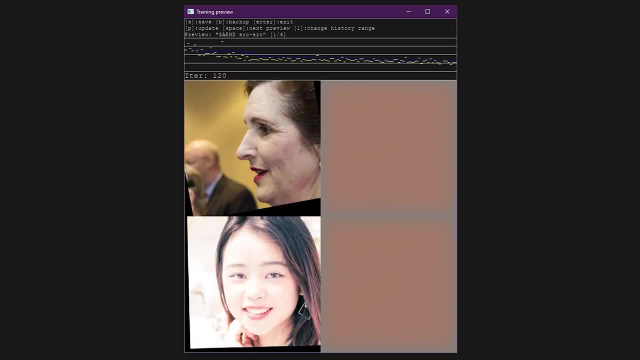 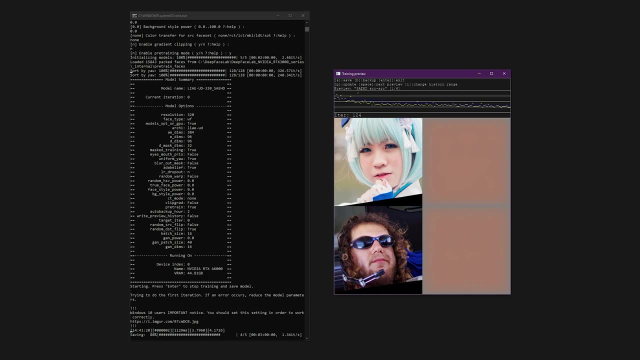 as the model reaches maximum accuracy, The L key changes the range history of the graph, which will have many thousands or millions of iterations. Once you have the pre-training running, you should consider raising the batch size for faster training. With the preview window selected, hit enter to save and stop training. 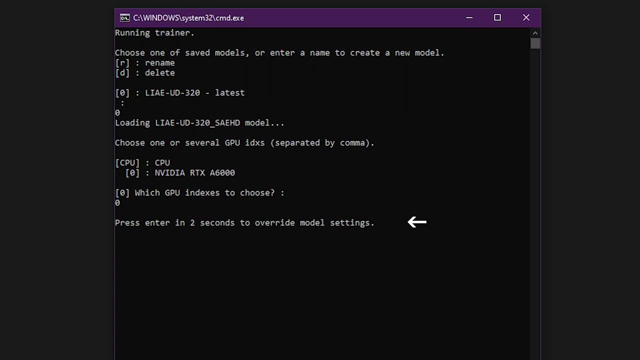 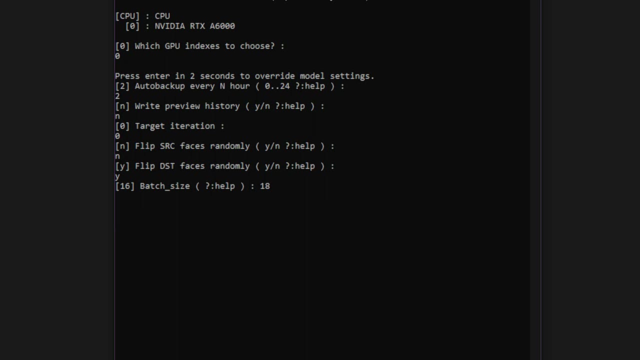 Run the trainSAEHD script again and this time hit enter when prompted, before the trainer starts. Now you can modify some of the settings, such as the batch size. Raise the batch size by one or two points and for the rest of the settings, just hit enter to keep the same values If the 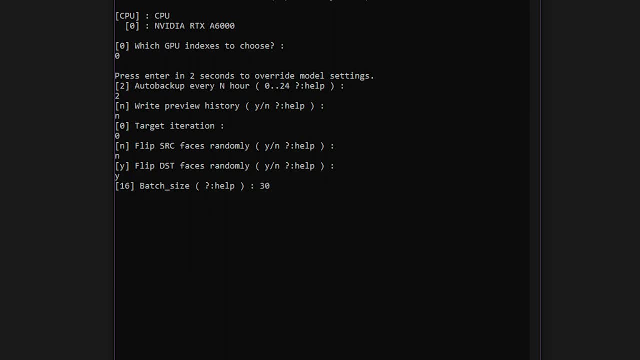 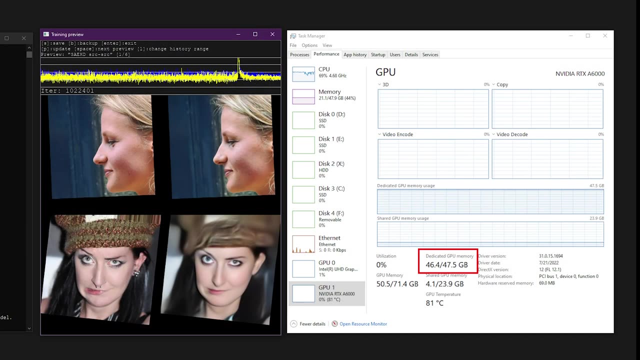 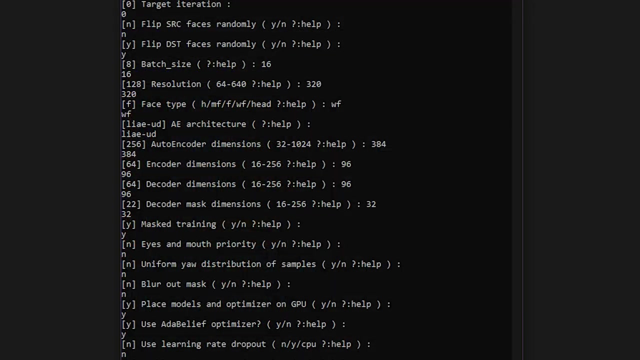 trainer runs, stop it and raise the batch size again. Keep raising it until the trainer crashes and you get an OOM error. then back it off by one or two points. Now you should be training at the fastest rate your system can handle, given the other model parameters you entered. If you can't, 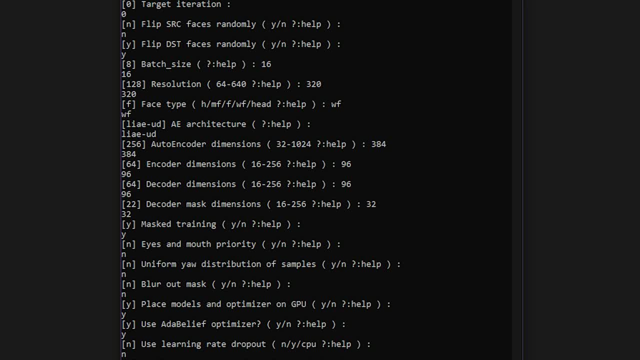 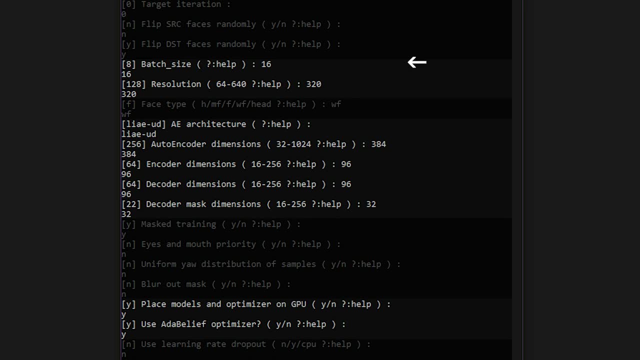 run the model, you're going to have to modify some of the values we entered previously. Enter all of the same settings again, but this time use a lower batch size If you end up having to lower the batch size to 4 or less. you can use a lower batch size If you end up having to lower the batch size to 4 or. 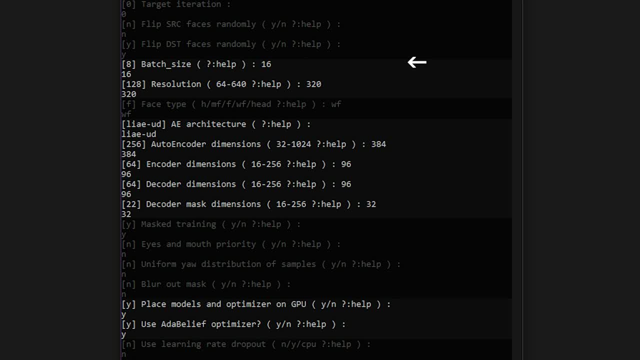 less, then that is a good indication that you need to adjust the other model parameters. Try it with Add a Belief disabled or use LIAE instead of LIAE-UD. You can turn off Opton GPU to free up some VRAM, but you'll probably be using more CPU resources during training. 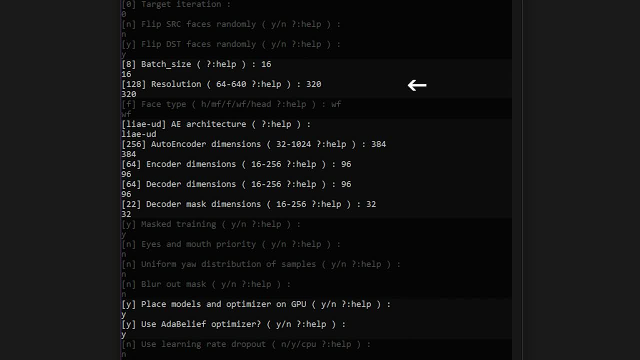 and the speed will be slower. Lowering the resolution will have a dramatic impact on the VRAM usage but of course, will affect the final quality. You can also lower the various autoencoder dimensions while keeping the same ratio between them, If you get any other errors. 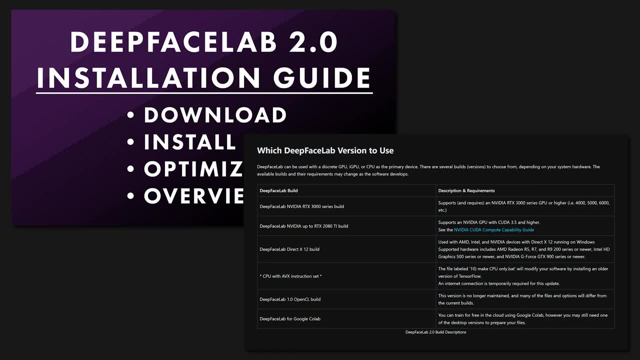 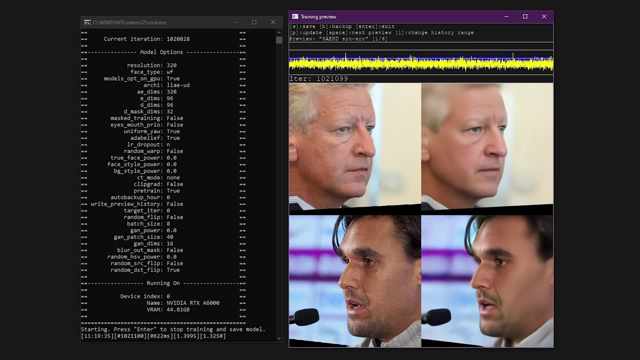 they may be due to using the wrong version of DeepFaceLab or that you need to optimize your system. Check out my DeepFaceLab installation tutorial video and my full guide at deepfakevfxcom for more tips on getting set up. At this point, you're probably wondering how long to pre-train. 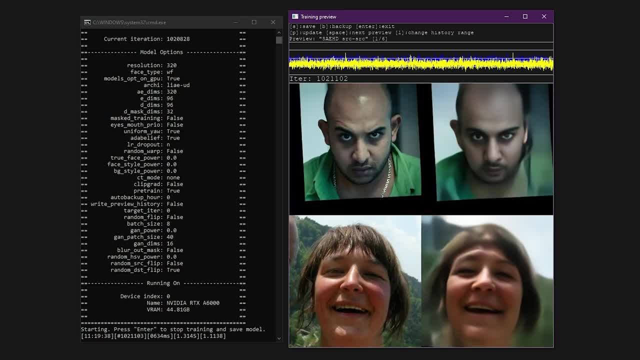 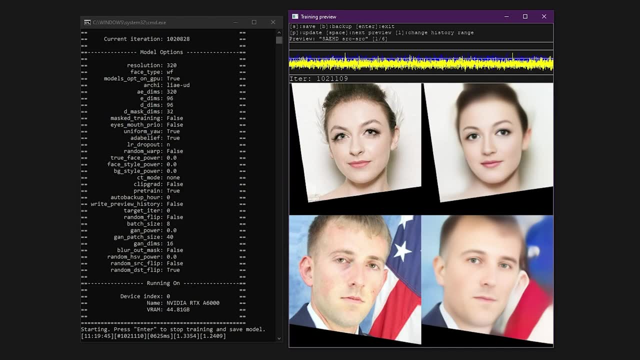 the model. Since there is no way to define how long a DeepFake model should be trained, you will use the loss graph and pre-train the model. You can also use the loss graph and pre-train the model Once the graph flattens out and the trained faces look similar to the original images. 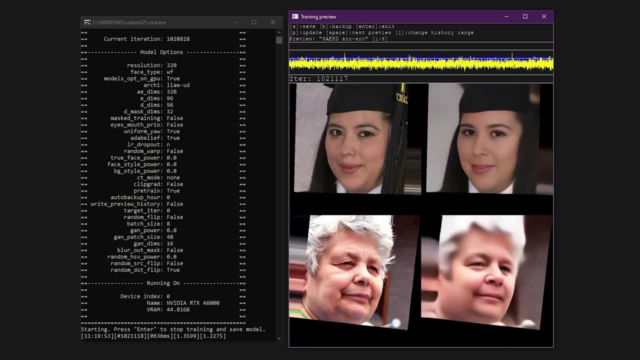 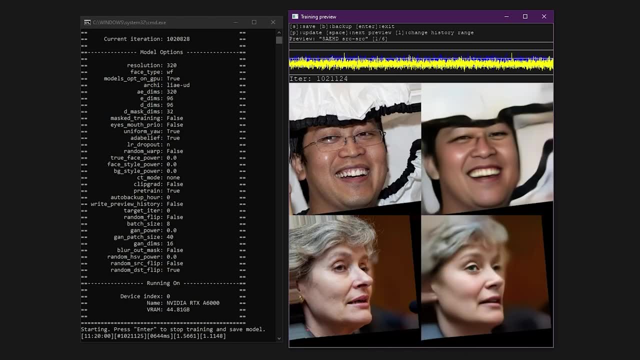 you can save, backup and exit the trainer. Remember that you can continue pre-training at any time, which means that you can use the model for a DeepFake right now and come back to it later on. Go to the model folder backups and save a copy of the most. 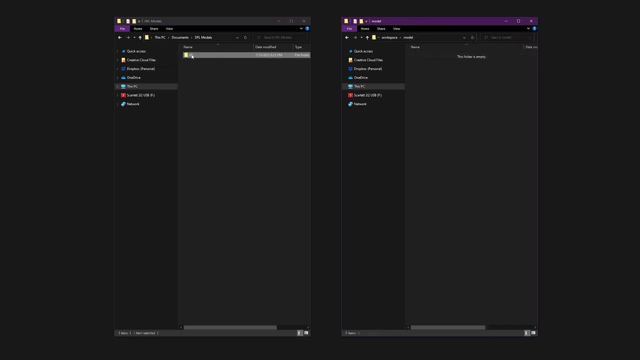 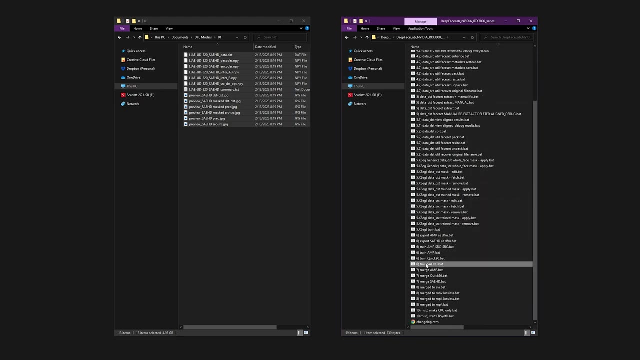 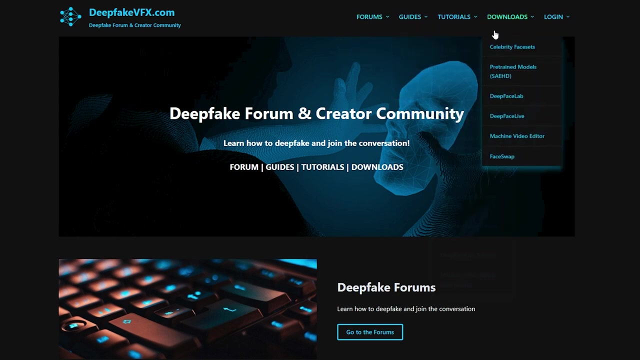 recent folder, usually number 1.. When you want to continue pre-training, simply drop these files into the model folder and run the SAEHD trainer again. If you have a pre-trained model you'd like to share with the community, log in to deepfakevfxcom, where you'll be able to download pre-trained models. 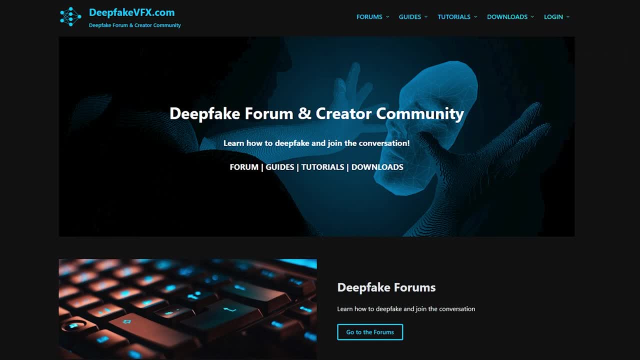 and submit your model to be listed in the archive. If you liked this video, help me out with a thumbs up and, as always, thanks for watching.